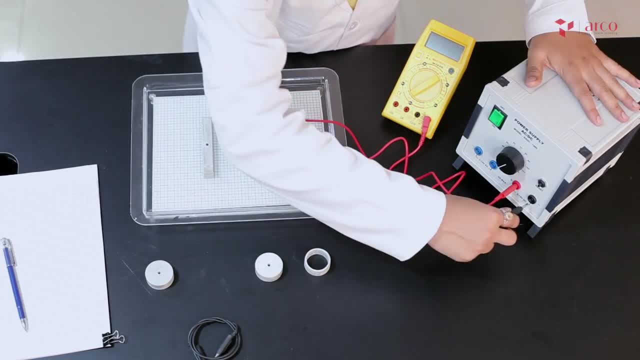 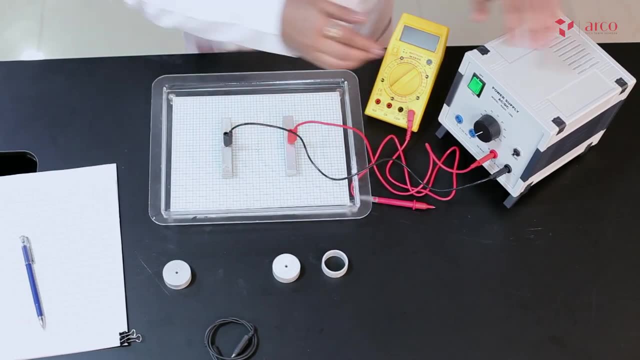 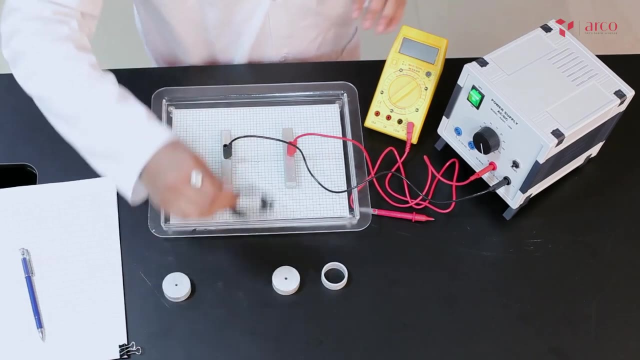 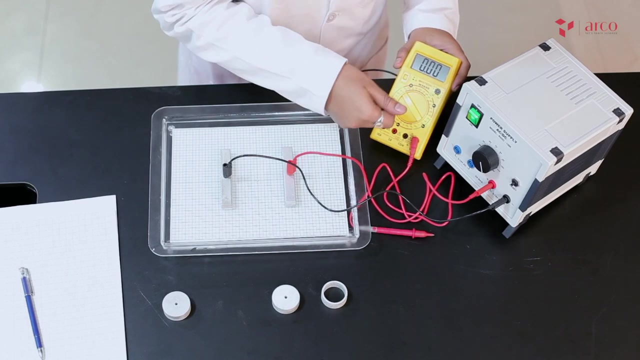 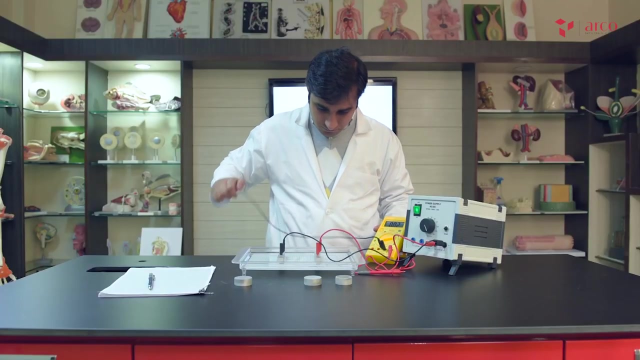 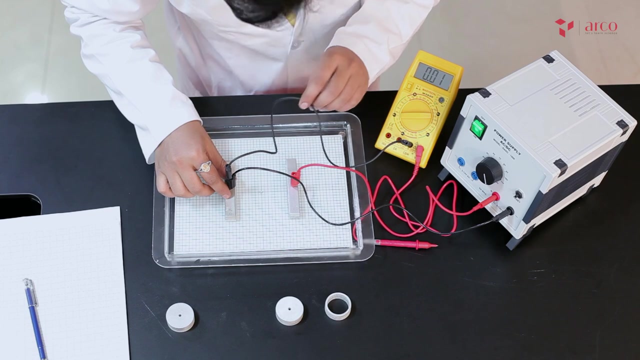 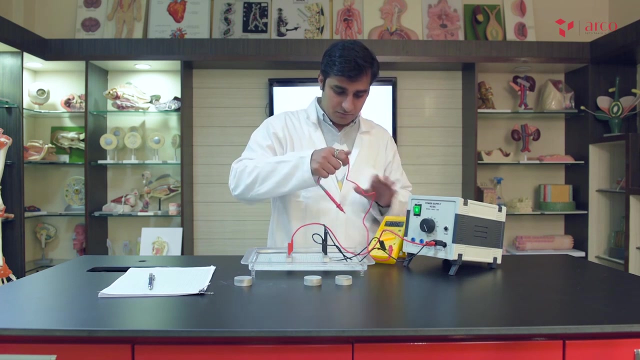 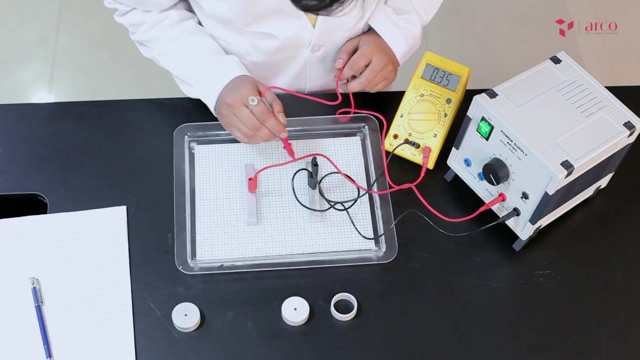 Now we will connect a multimeter in voltage mode across these bar electrodes placed in saline water and check the output voltage on the positive electrode as well as on the negative electrode. As you can see, the positive electrode is showing the voltage approx. 12 volts per second. 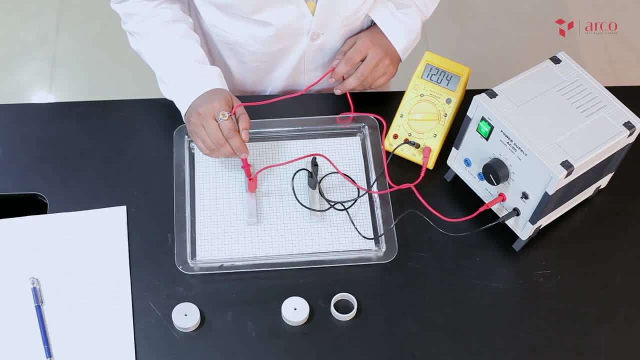 The negative electrode is showing the voltage of 0 volt and the exact center of these electrodes will show the half of the set voltage from the power source, which approx 6 volts DC. To check the center and the steps from negative to positive electrode, a graph is printed. 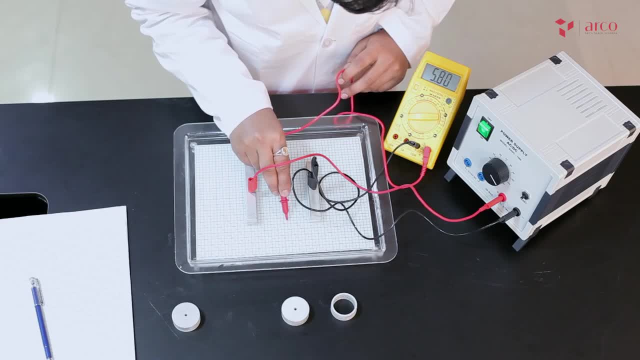 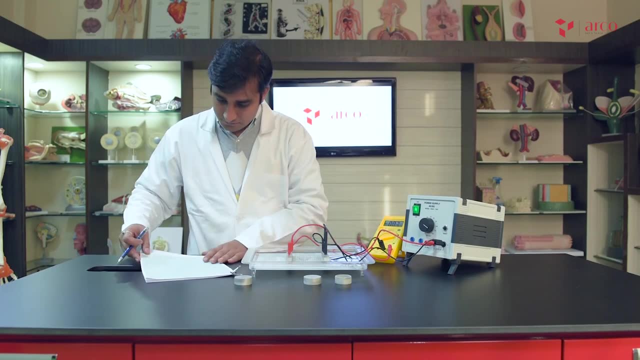 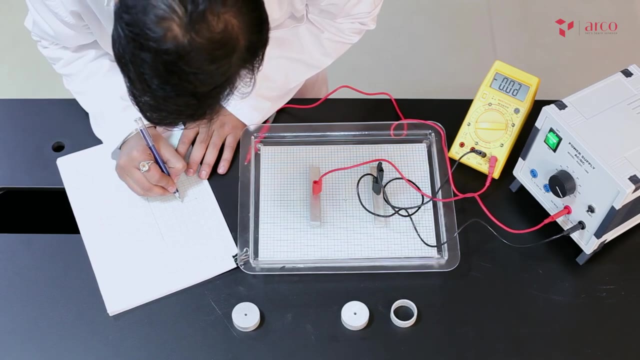 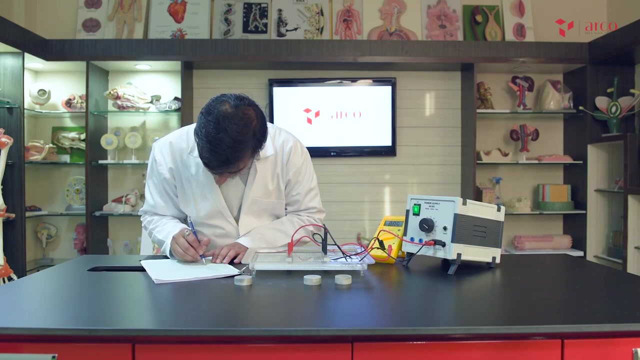 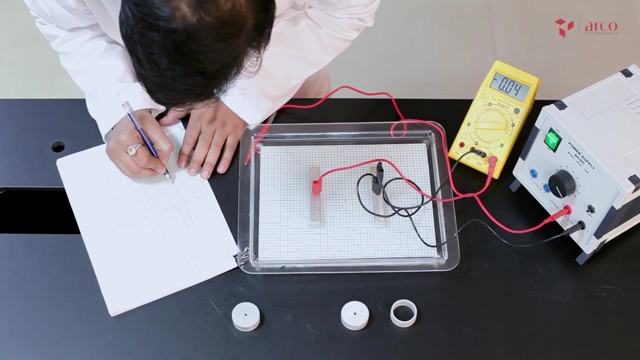 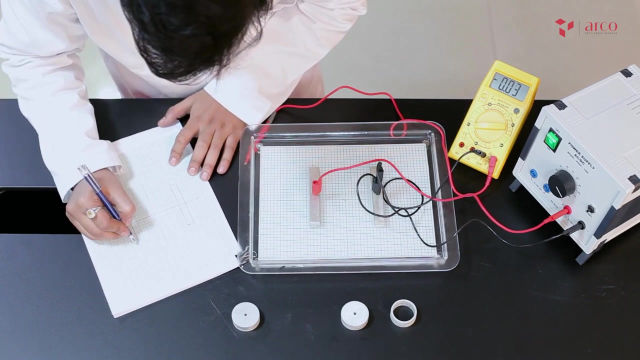 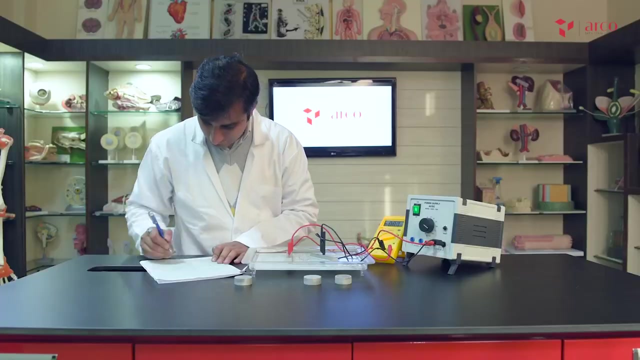 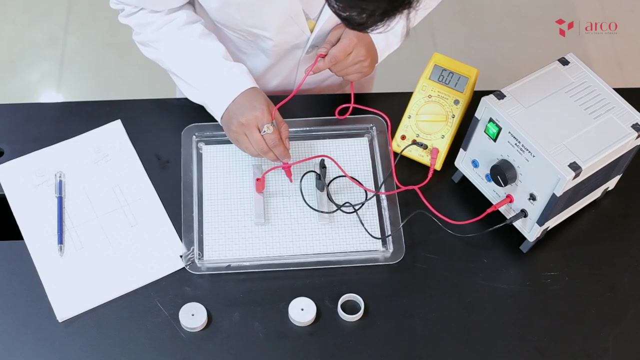 on the top It is complete straight center line parallel to the electrode will show the constant voltage. Now we will draw the same waves on graph papers simultaneously, which we will observe in the trough. We will observe the field lines from 0V to 12V and draw the same on the graph paper. 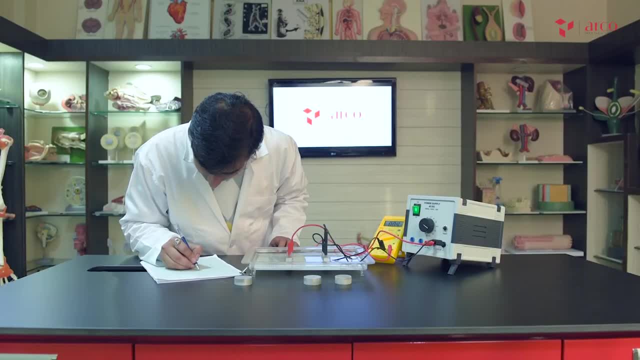 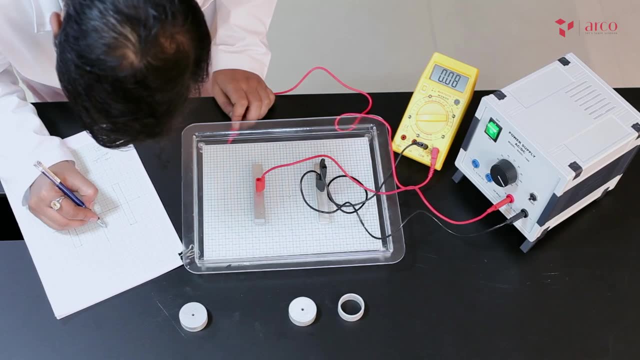 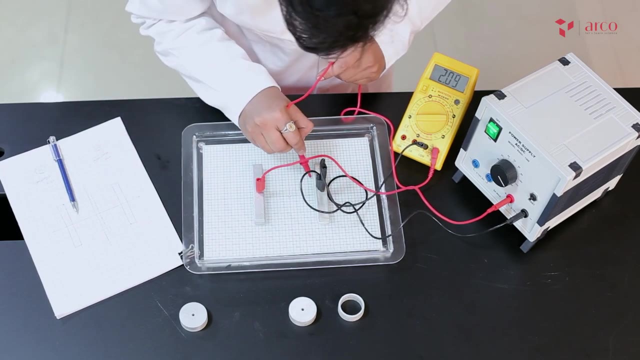 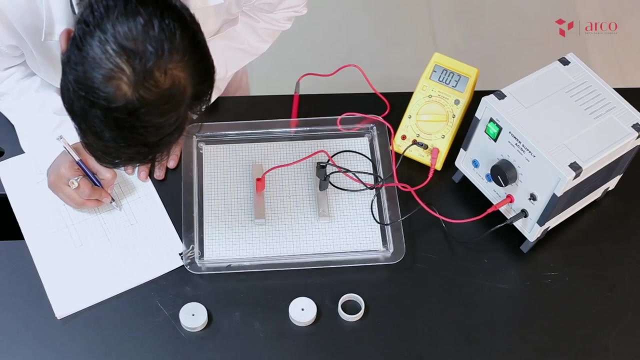 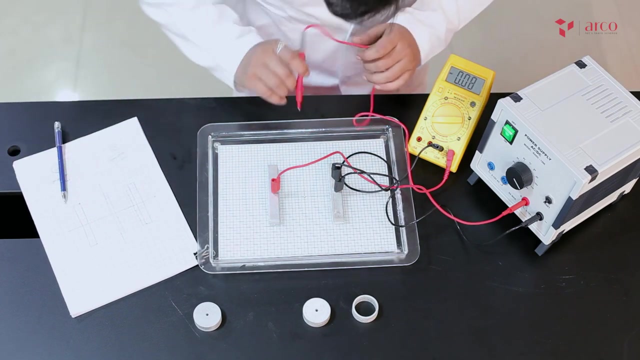 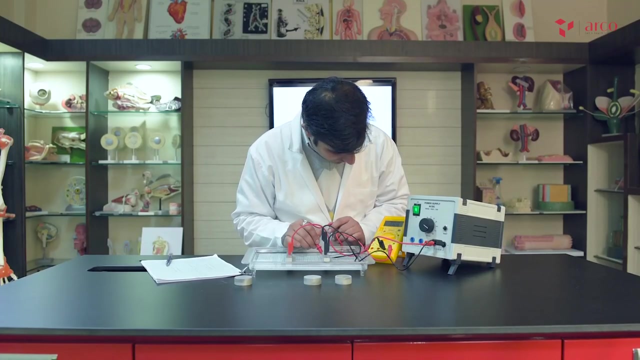 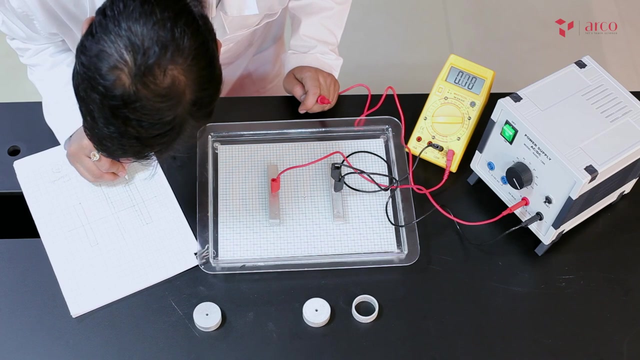 We will find the line of a 12V perox near the negative electrode and observe the same parallel to the electrode. Also observe the same at the concern of the electrodes. We can observe that these lines are getting turned in curves and we will draw the same. 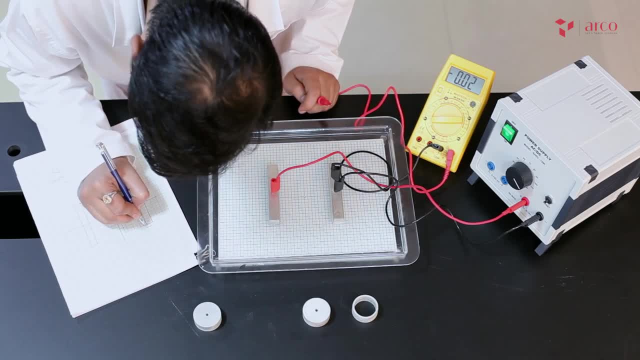 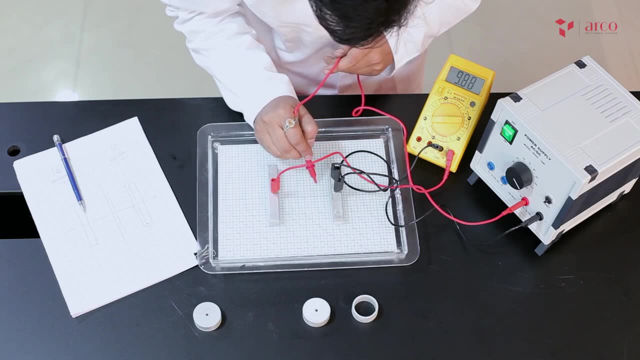 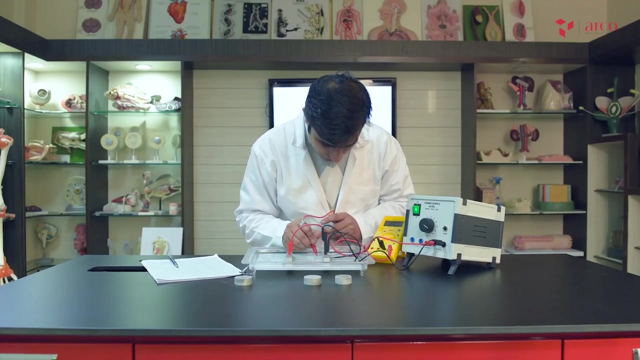 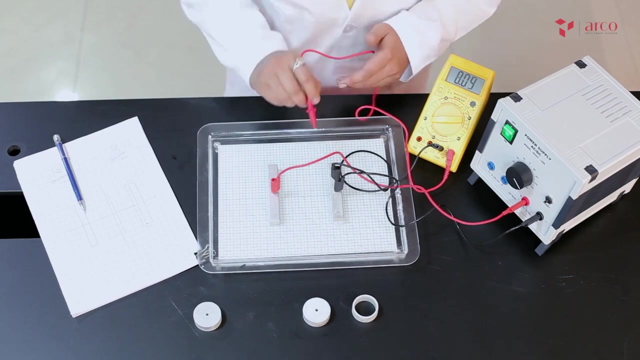 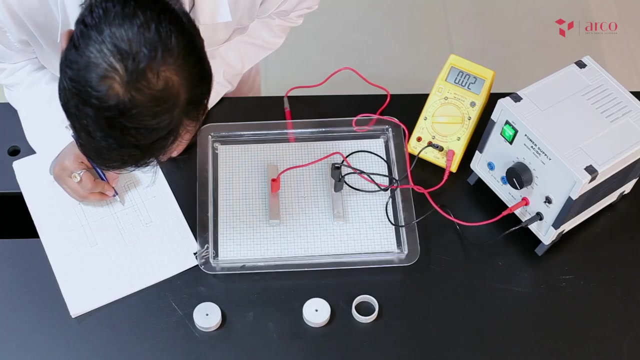 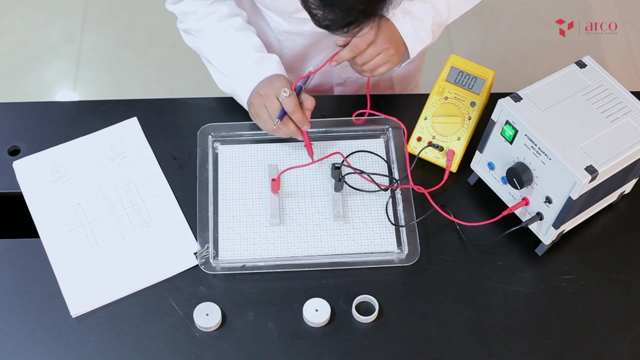 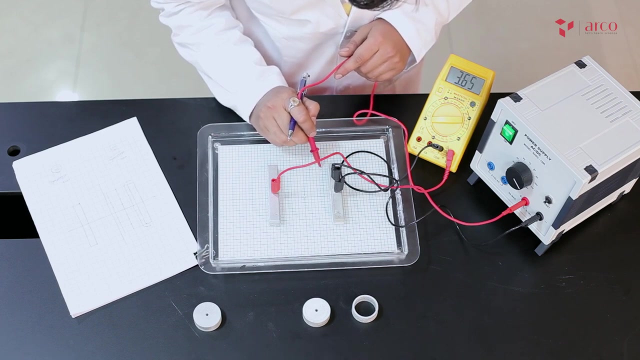 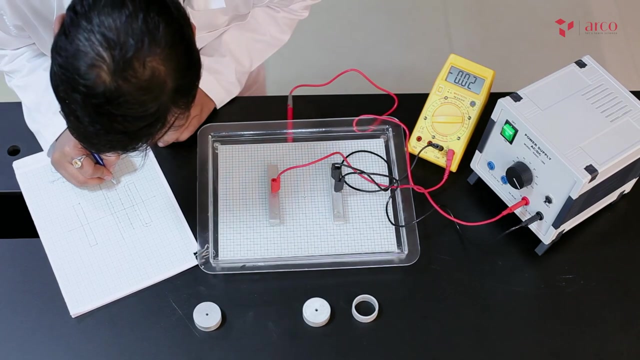 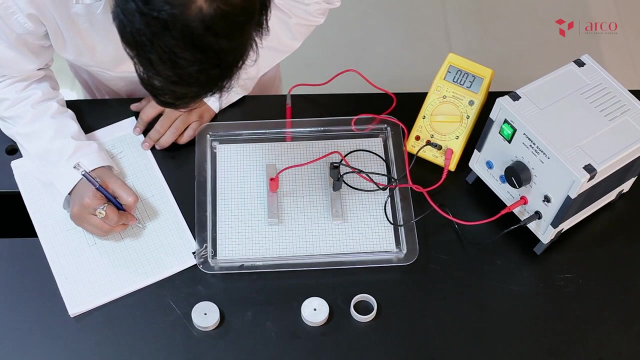 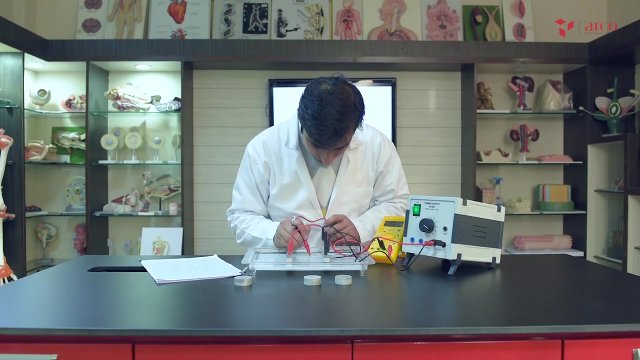 on the graph. Now we will repeat the same procedure for 4 volts and draw the lines on the graph paper as observed in the trap of saline water. We will repeat the same procedure at every step of 2 volts. 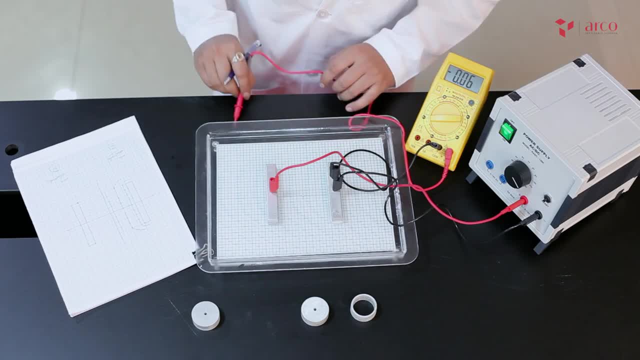 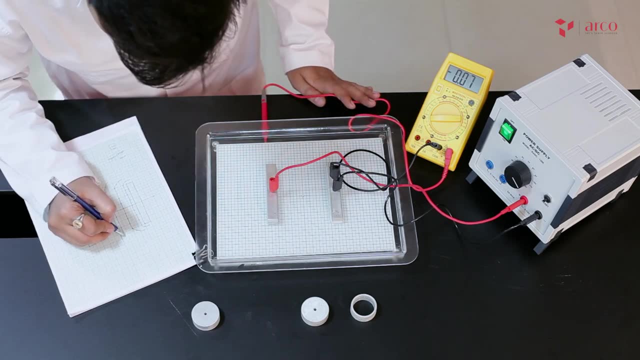 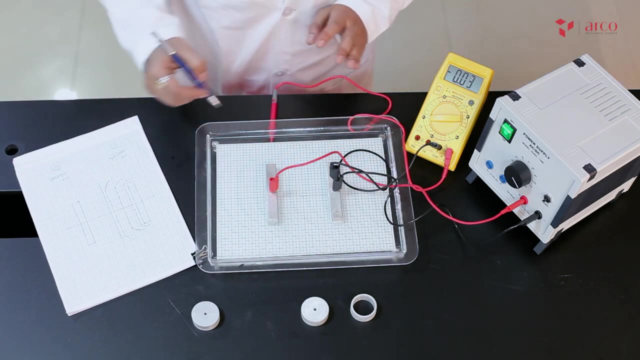 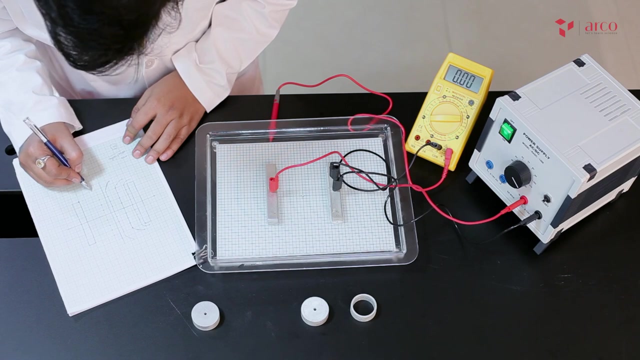 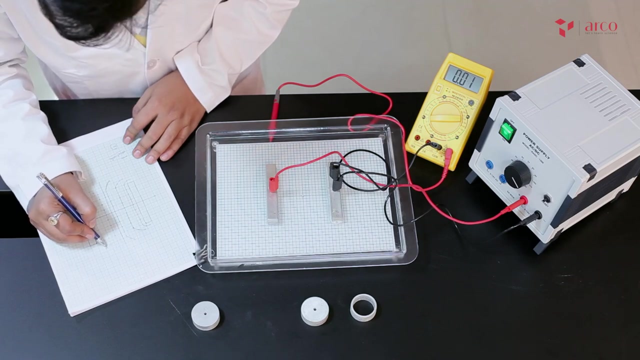 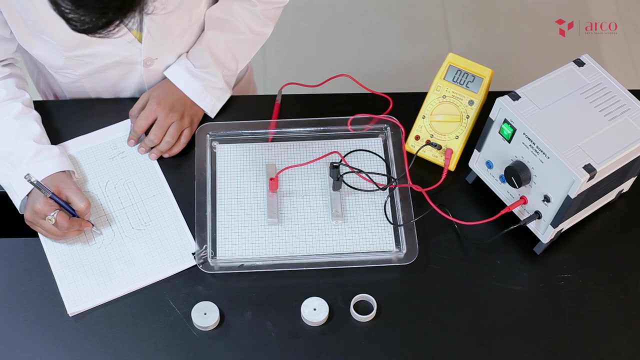 We will repeat the same procedure at every step of 3 volts, from 0 to 12 volts, and draw the lines on graph papers as observed in trap of saline water. Next, we will repeat the same procedure and the same guessing process at the end. 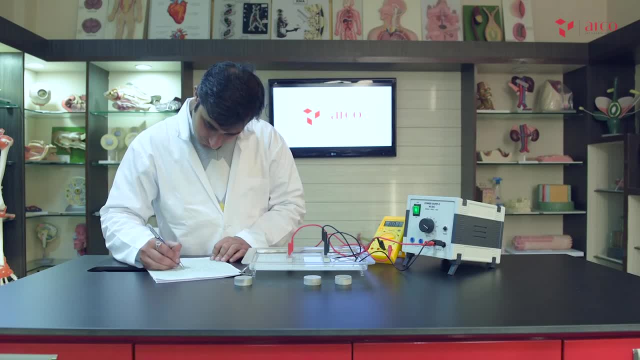 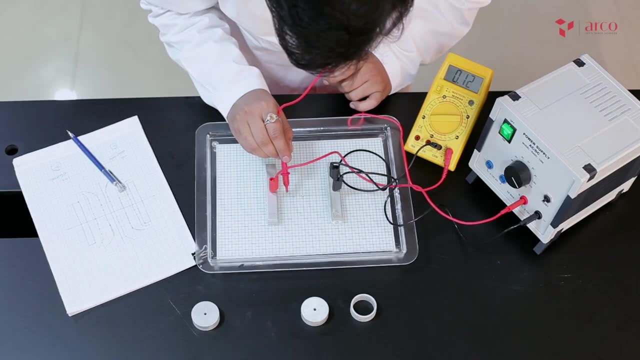 We add the new tip of the不到 mixed wealthyあぁ ingredient And we measure the new tip of the Alright ingredient using pionastry draw brush. Done Thanks for watching. See you next week signing off. Bye, Bye.